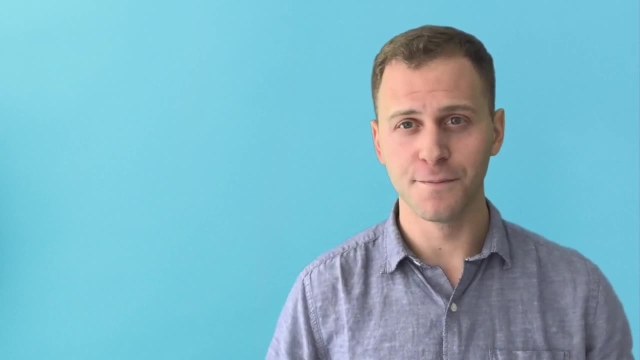 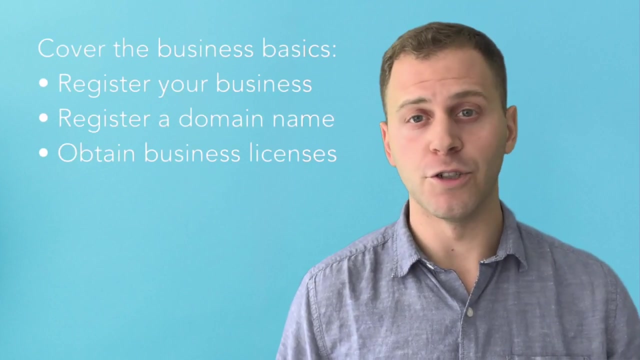 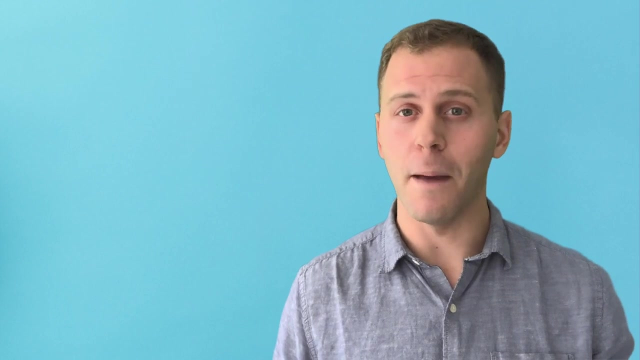 Here are the six steps to starting your own import export business. Step one cover the business basics. This means registering your business with the state where your headquarters will be located, registering a domain name, getting any business licenses you need to legally operate, and so on. You'll need a business plan too. Part of that business plan. 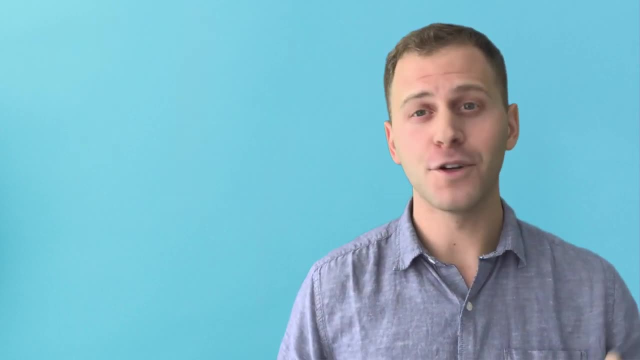 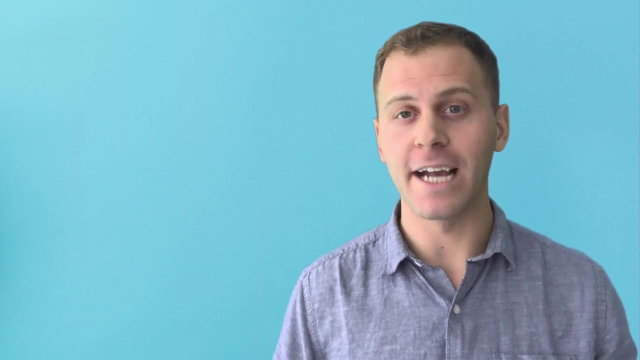 needs to cover the rules and regulations of the markets you want to work in. For example, to bring alcohol and tobacco products into the US, you need, yes, an alcohol and tobacco trade and tax, which can take months to acquire. Similar research needs to be done when doing business with other. 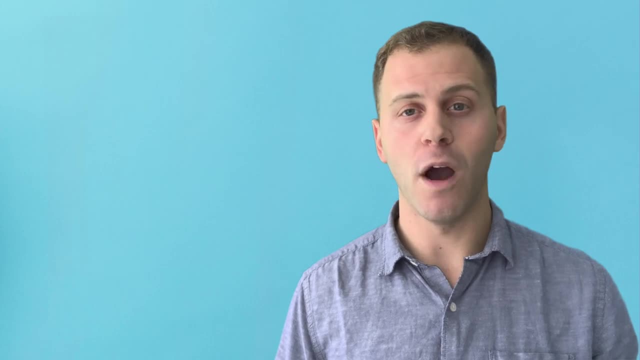 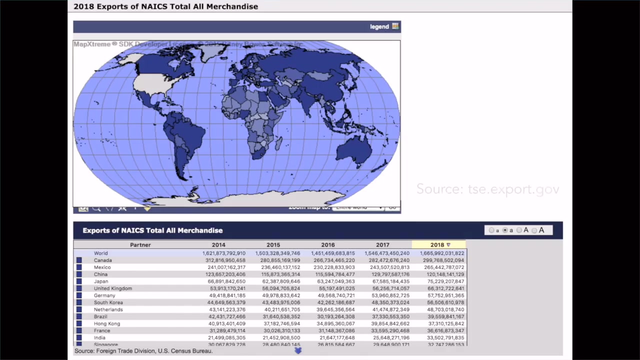 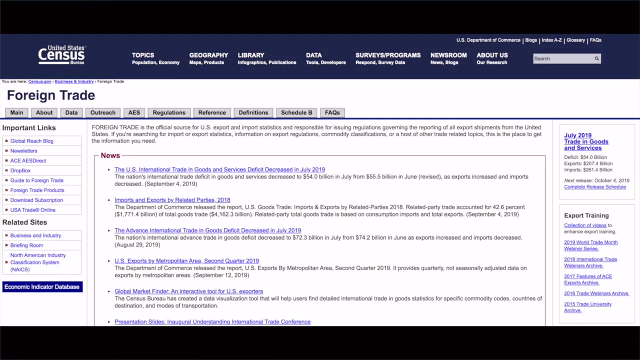 countries, covering everything from legal back label requirements to insurance. You can conduct research with resources like Global Edge's Market Potential Index or by checking with local government officials and websites such as the Department of Commerce International Trade Administration's data and analysis. You can also find reports on the state of the imports exports. industry with the Census Bureau's foreign trade page. Perhaps most importantly, you need access to capital. Startup costs can vary greatly depending on the type of imports- exports business you want to start. Everyone knows it takes money to make money, so it's helpful to 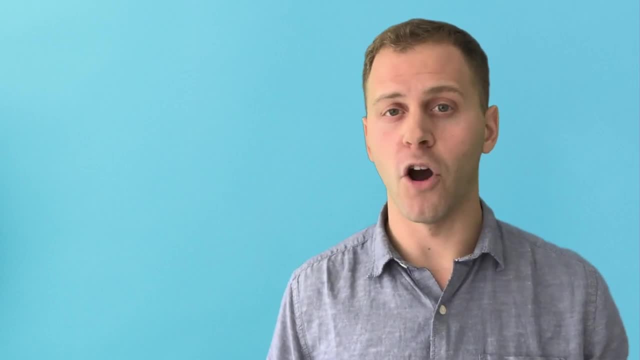 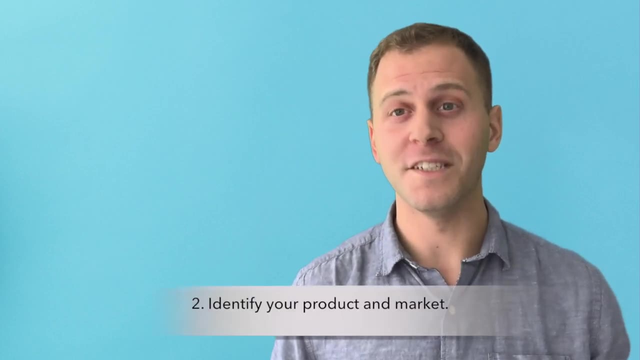 have capital on hand when you're getting started. Look into a business credit card with a 0% introductory APR offer, if you qualify, or a startup loan or line of credit to get you going. Step two is identify what you'll import or export, as well as your market. This step goes right along. 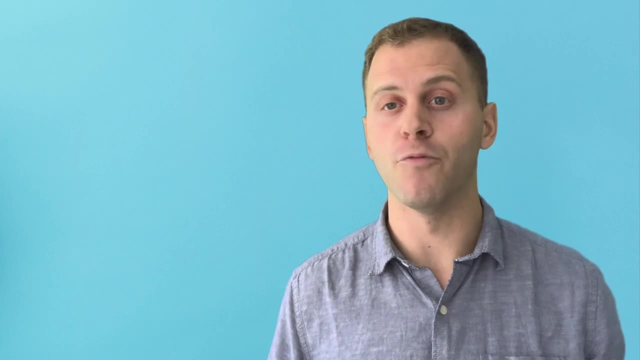 with step one, because, in order to write your business plan and understand what regulations you'll need to follow, you'll need to know what you're going to need to follow. You'll need to know what your importing or exporting is. If you're getting into this business, it's either because you have 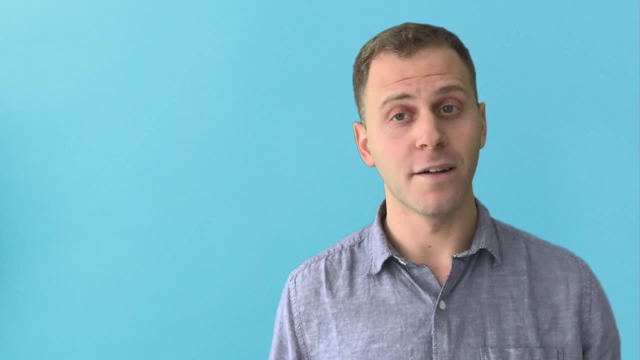 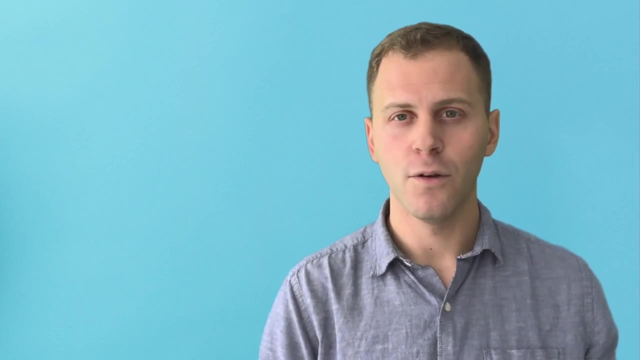 a passion for international business, or you've identified a product that would shine in another market, or both. So let's assume the former reason is your reason for getting into this business. What are you going to export from your home market to another? Maybe it's wine from South Africa to? 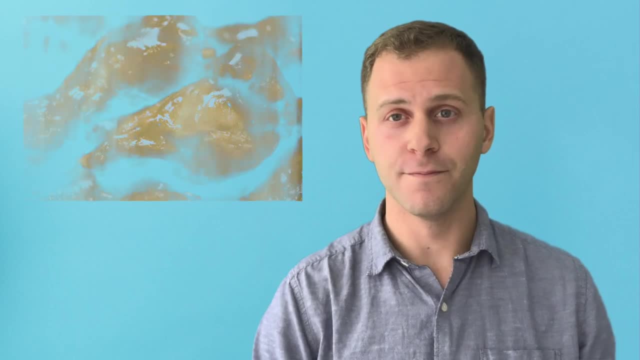 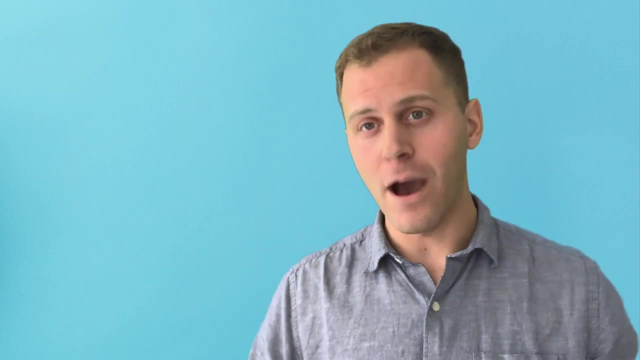 the United States or buffalo wing sauce from the US to Europe. You'll typically want a deep familiarity with both: the product you want to import, export, the market you're targeting, or both. That's a great way to understand the value proposition of what you're selling and any jargon or industry. 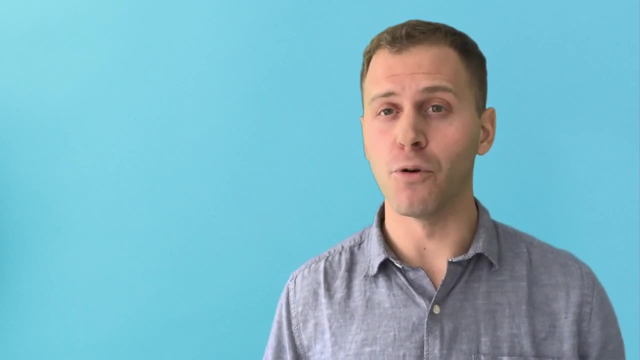 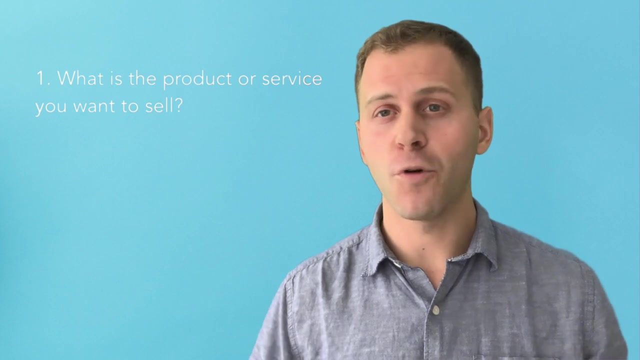 or market specific talk that will help you stand out in a crowd of other importers and exporters. Market research is a big undertaking, but the basic questions you'll want to answer include: number one: what is the product or service you want to sell? Number two: who is your target? 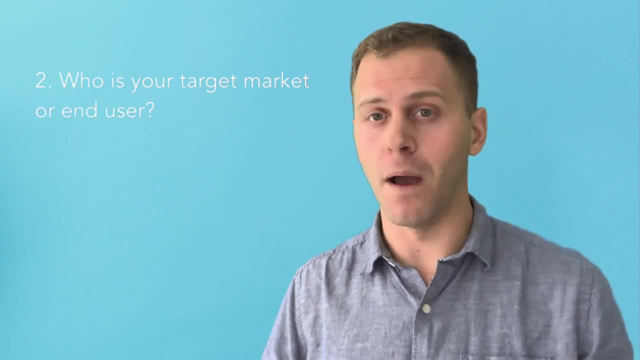 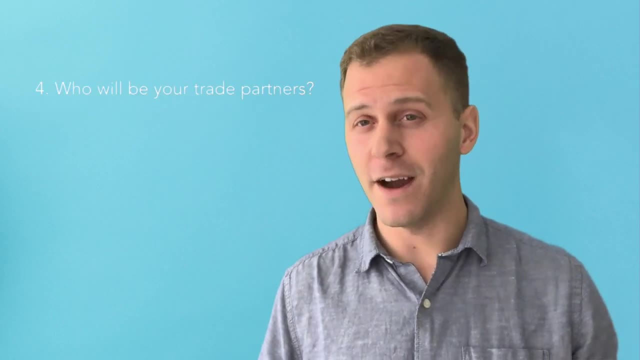 market or end user? Is it the mass market consumer or for use by businesses or governments? Number three: what country or countries will you import from or export to? And number four, finally: who will be your trade partners? your trade partners could be a manufacturer's representative. 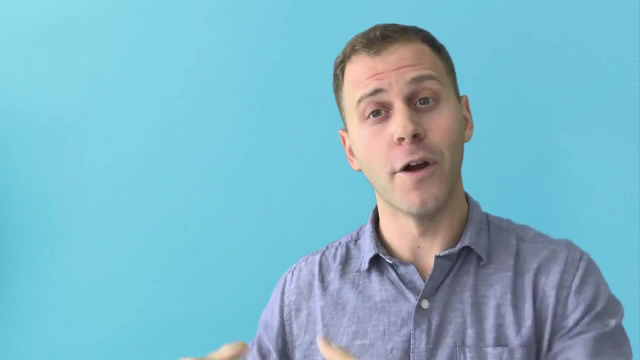 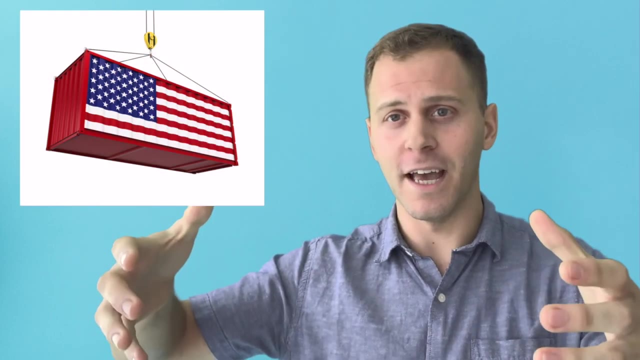 wholesale distributors or retailers on either side of the importing or exporting process. these are the people you'll deal with, so you're not just buying up caviar in france, putting it in a box that says usa and expecting someone to buy it when it hits the ports. step three is to 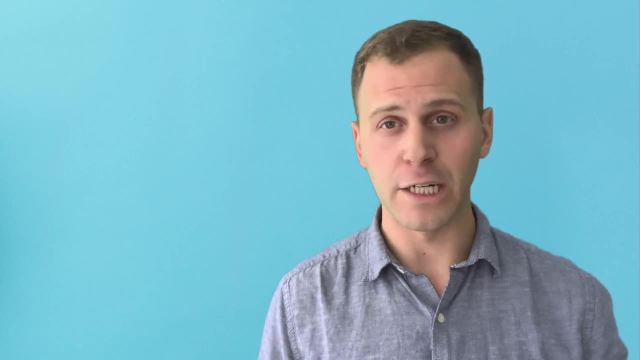 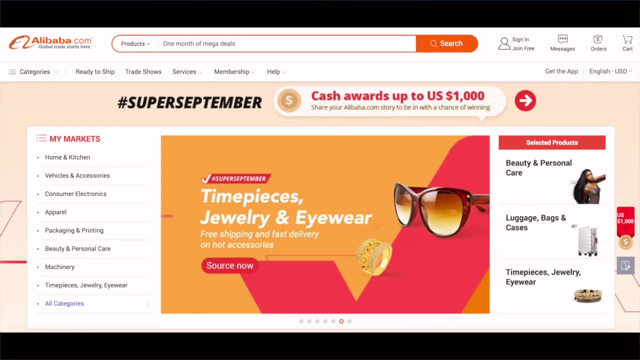 source your suppliers. when you get in touch with a wholesaler or manufacturer's representative, you'll already have a lead on a supplier for your product. generally, you can also find suppliers to companies like alibaba, global sources and thomas register. you can find links to those companies. 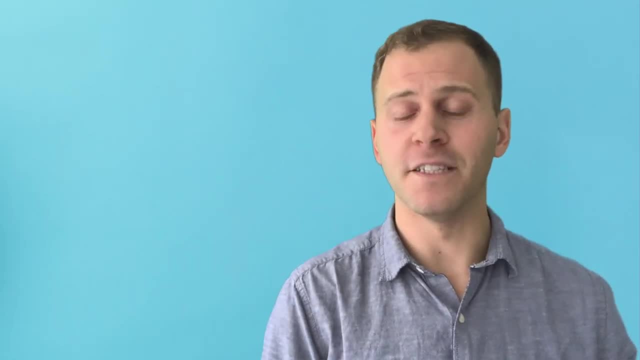 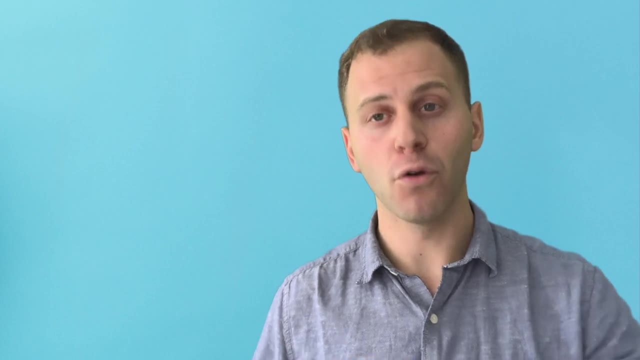 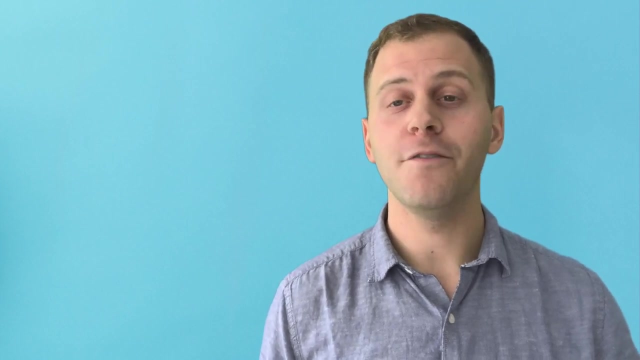 down below. you will need to convince your potential supplier of the benefits of entering the us market or another market if you wish to sell to that one and figure out the logistics of taking their product from their local warehouse or production facility to another one, potentially on the other side of the globe, maybe you'll become your own supplier. you can investigate what it. 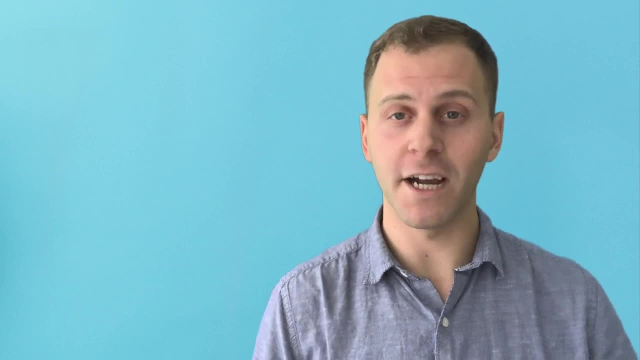 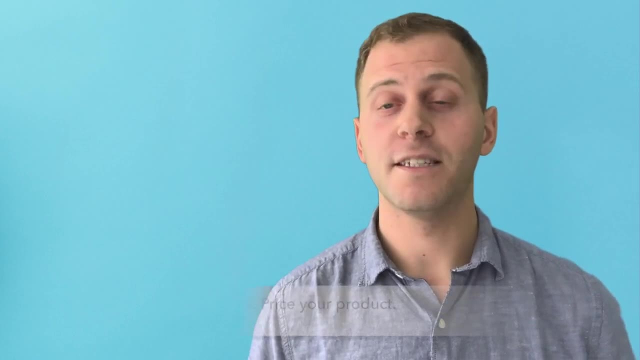 would cost to buy an interest in the product or service you want to import or export, giving yourself an added incentive to find an international supplier for your products and also to find an international home for the goods that you now have a vested interest in. step four: price your product. okay, you know what product you want to work with and you've identified. 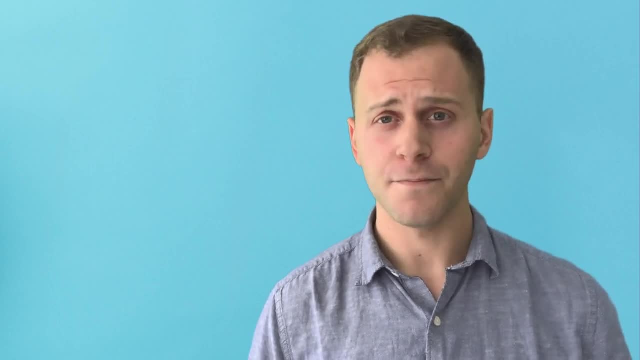 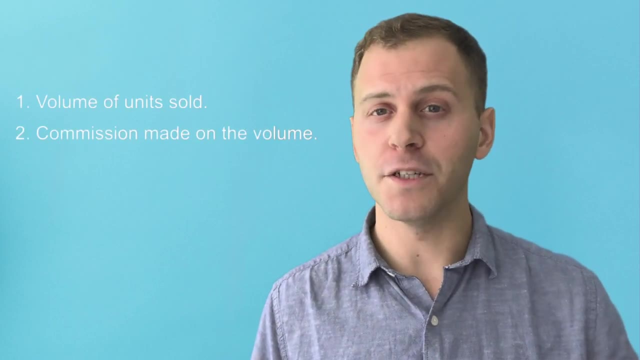 your target market next up, figuring out how much to charge. typically, the business model on an imports- exports business includes two key understandings: the volume of units sold and the commission you made on that volume. you might also get paid with a salary or flat retainer plus. 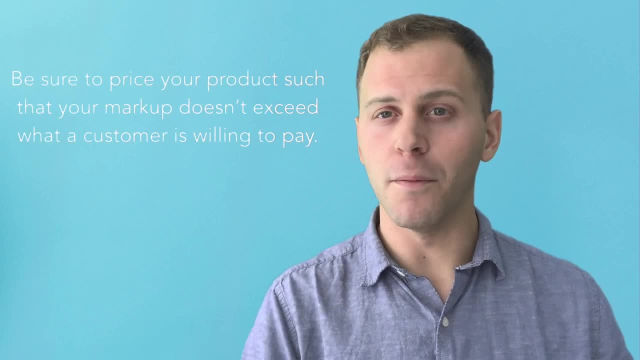 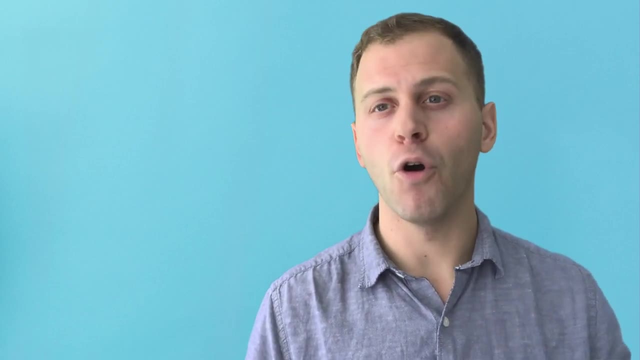 commission. if you're an emc, be sure to price your product. it doesn't exceed what a customer is willing to pay for it. but you don't want to make it too low so that you won't make a profit. your overhead and the specifics of what you're importing or exporting. its price, its cachet, its availability will play a huge role in dictating your price. of course, in this industry, importers and exporters typically take 10 to 15 percent mark up above with the manufacturer charges when you buy the raw product. step five is identify your customers. it's one. 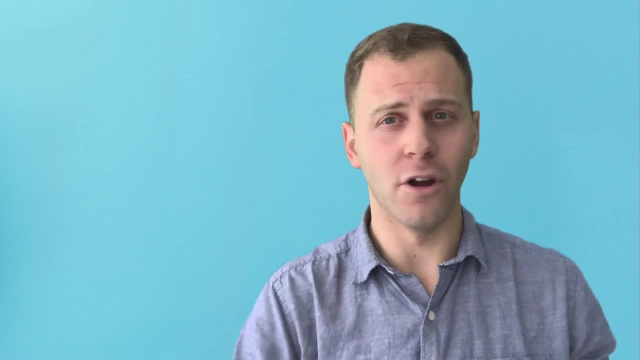 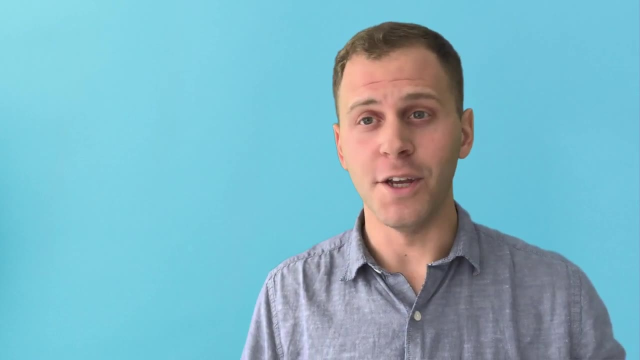 thing to have an idea of who your customers are or what your target market is, but it's another thing to actually get them on the line and have them agree to buy from you or sell to you again. you can't just send your products to the port of. 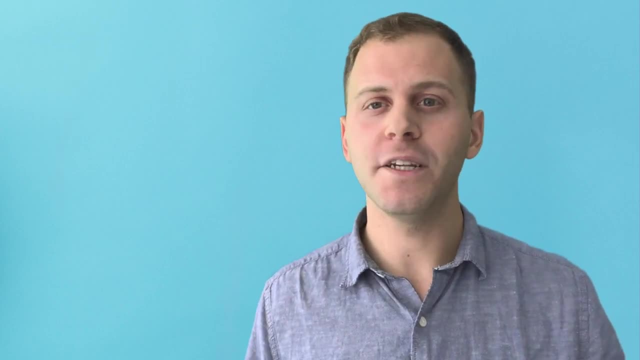 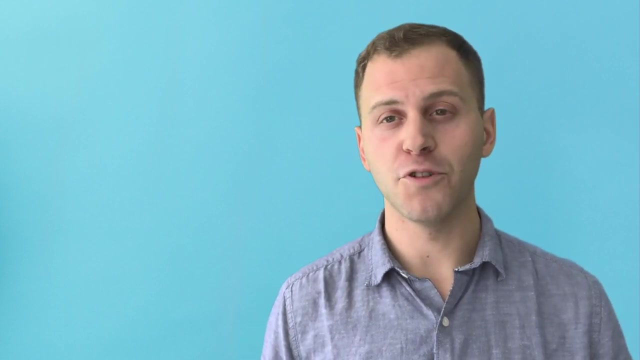 new york and start selling your wares to whomever walks by. you usually need to find distributors and clients, and there are a few ways to do that. if you have a quality website and you market it well, your customers may end up finding you. cold calling is also a time honored and useful tactic. 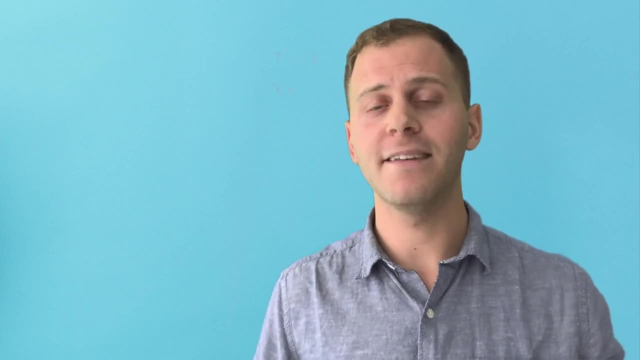 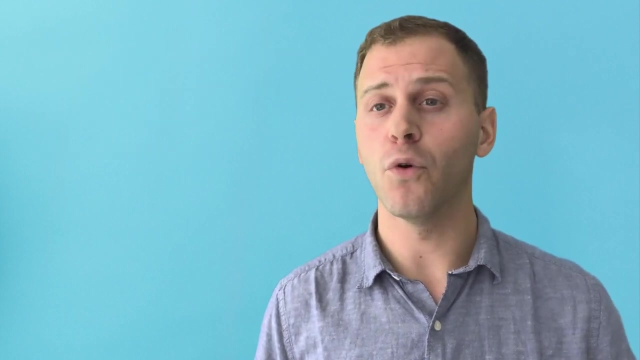 check with any local contacts you have in the area or contact the region's chamber of commerce, trade consulates, embassies and so on. these organizations and offices might be able to give you a local contact list that could be vital help in starting an imports and exports business. 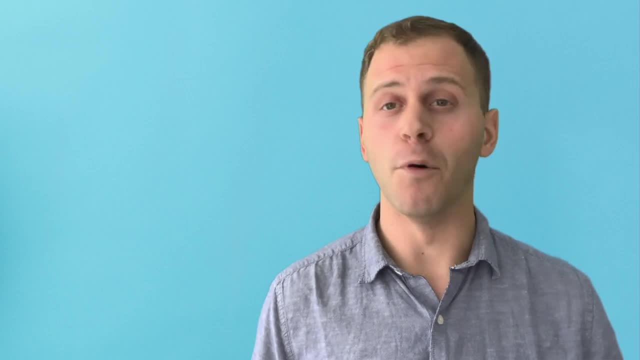 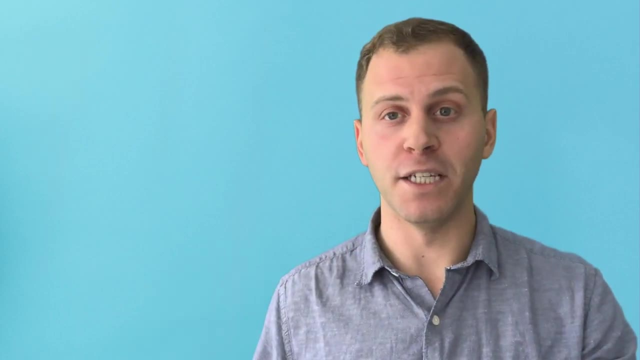 step six is finalize the logistics. this is your biggest and most complicated step, and the one that covers a variety of bases, from finalizing your supply chain to potentially moving into an office space. if you started out as a home-based business, this step will also be markedly different, depending 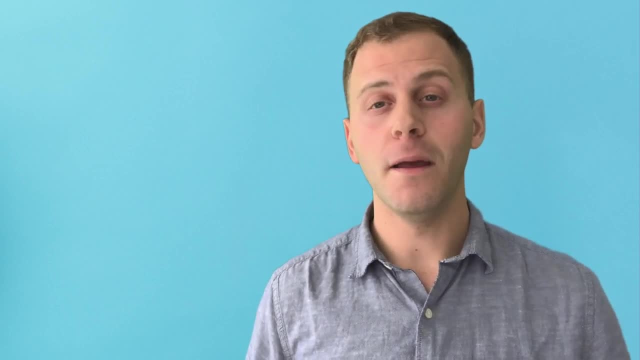 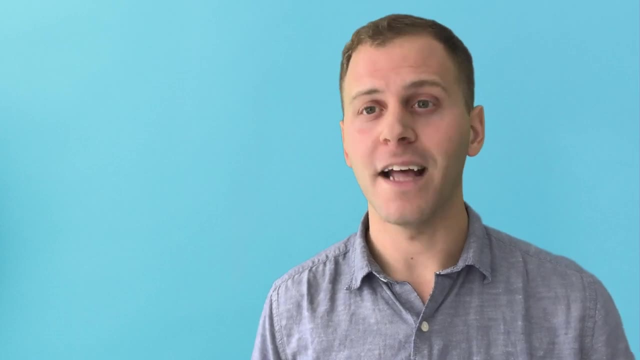 on what kind of import export business you decided to start. if you're an import export merchant, you may want to get in touch with a global freight forwarder to serve as a transport agent for moving cargo. that saves you a lot of time and worry about getting your products from the factory. 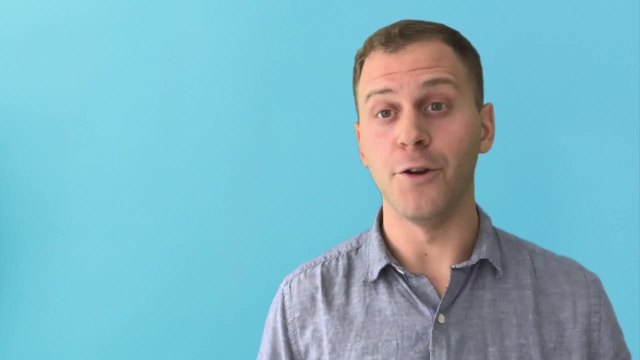 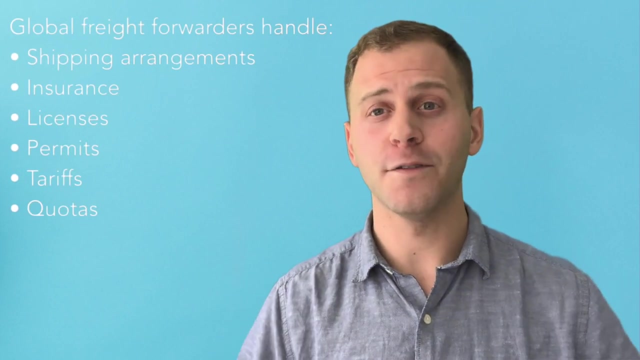 to a warehouse. you'll give them information about your business and your intentions for the product and they'll arrange the shipping agreements, insurance and even the licenses, permits, tariffs and quotas of working within another country- if you're an emc or etc. you might do all these. 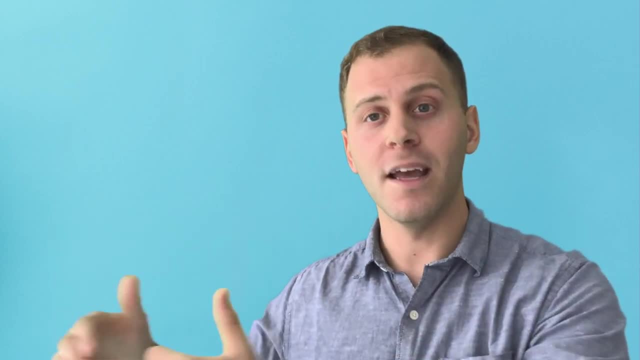 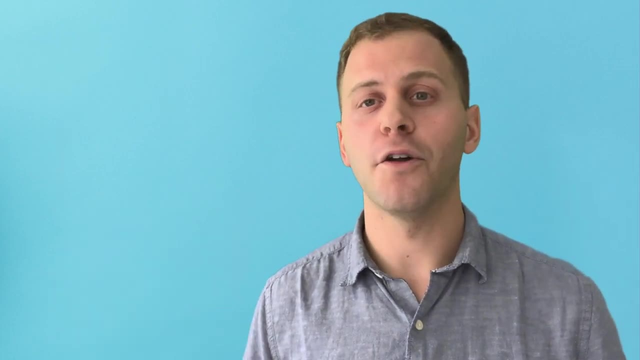 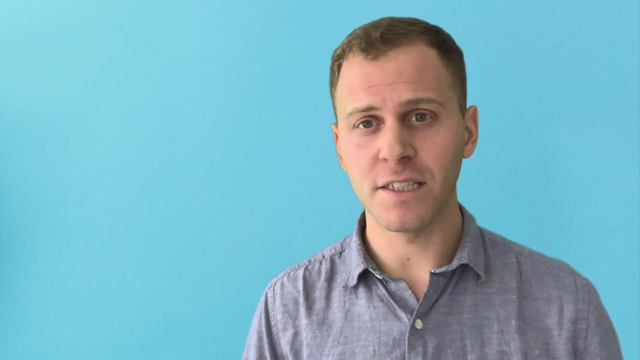 processes in-house and need to worry instead about putting money and time towards marketing your services or renting out commercial office space as your operation grows. essentially, you need to start thinking about importing and exporting as a business, not just as a series of transactions, and make sure that you're taking all the steps necessary to remain profitable in. 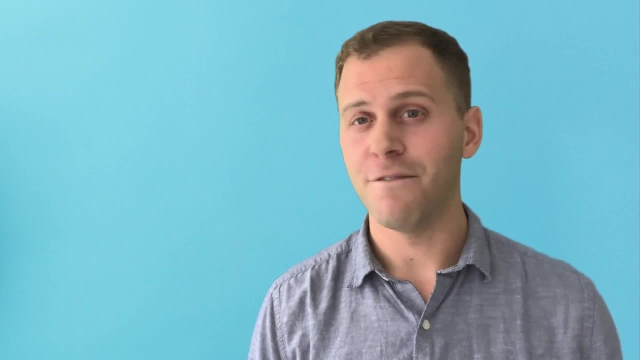 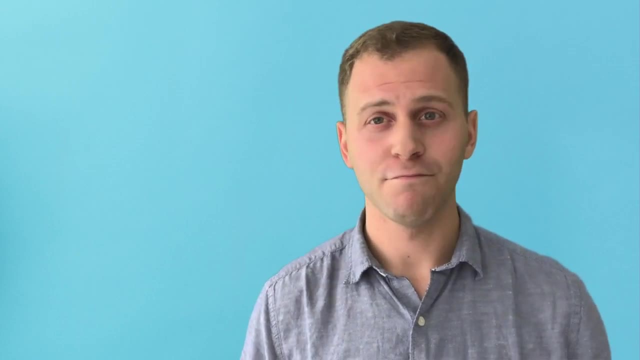 the months ahead. joining an import export association, finding a mentor in this space and getting in touch with local and federal government agencies will be a huge help in making this happen for you all. right, that about covers the basics of starting an import export business. it's a complex topic. 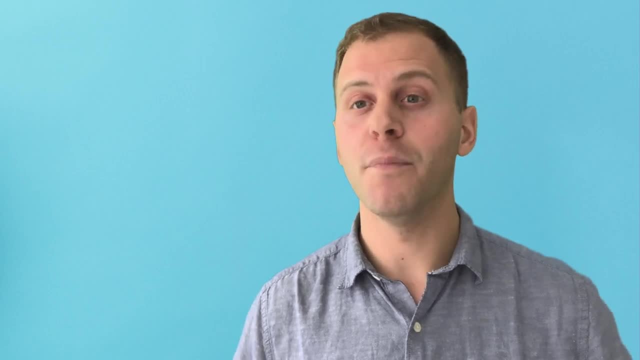 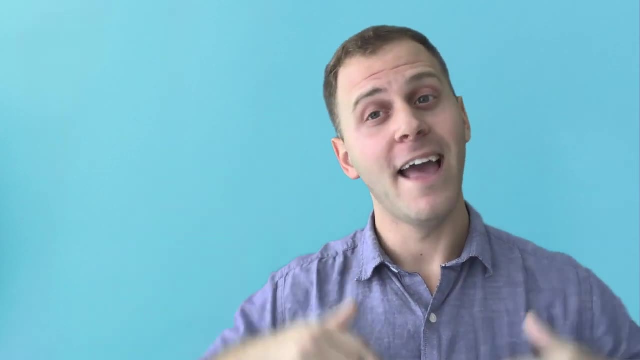 that requires a ton of research and hard work, but the thrill of making your services a part of the framework of international trade can make it all worth it. let us know if you have any questions or comments down below and, of course, subscribe to our channel for more insights into.